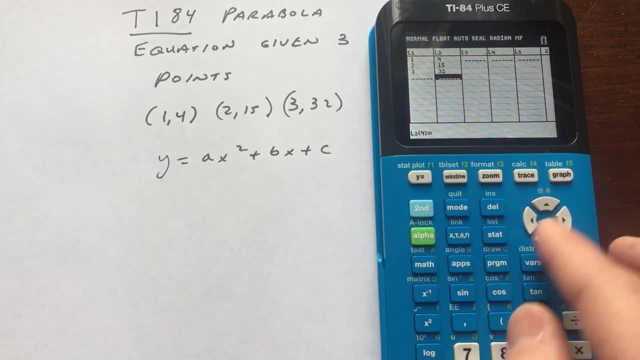 so you can see the points there: 1,, 4,, 2,, 15,, 3, 32.. Then what you want to do is you want to go back into stat- okay for statistics. You want to arrow over to calculate And you want to head. 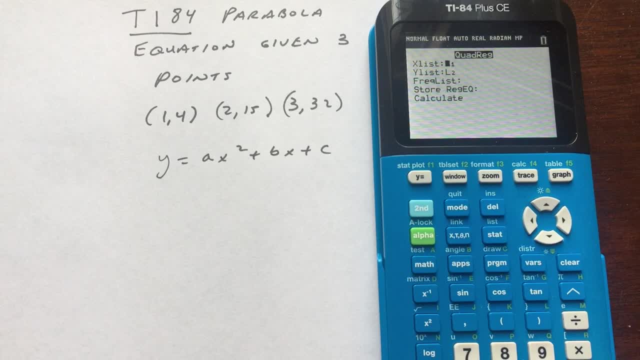 down to quadratic regression number 5.. I'm pressing enter And then what you want to do is you want to arrow down list 1,, list 2,, all the way to calculate, And then press enter one more time And you can. 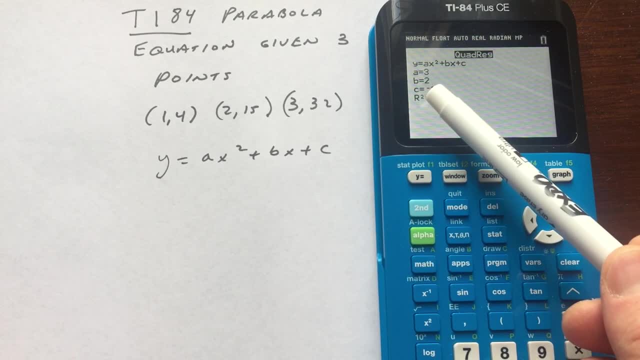 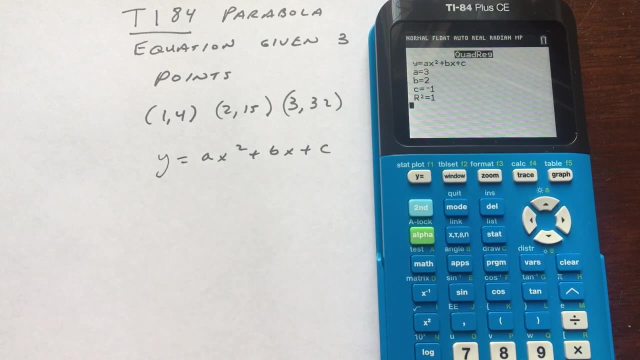 see what it's doing is it's giving you the a value, Which is 3., The b value, which is 2. And the c value is negative, 1.. You just have to substitute those in for a, b and c And you've got the equation of your quadratic right here. So if I 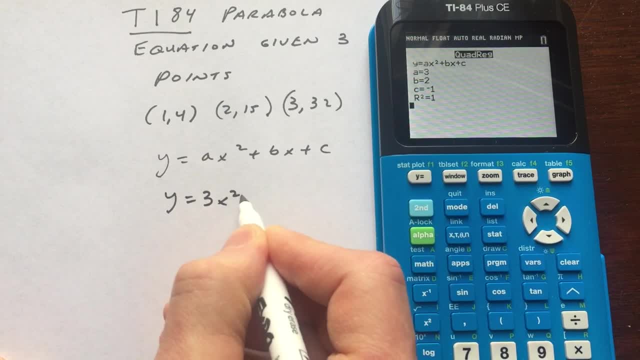 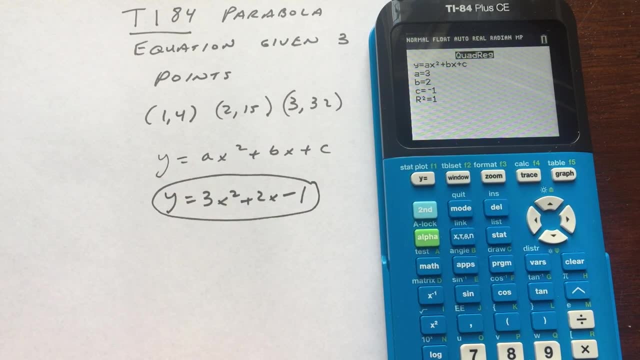 was to write it. it comes out to: y equals 3x squared plus 2x minus 1.. And that's your equation. So if you enjoyed this video, take a look at some more of the TI-83 and TI-84 videos that I did on. 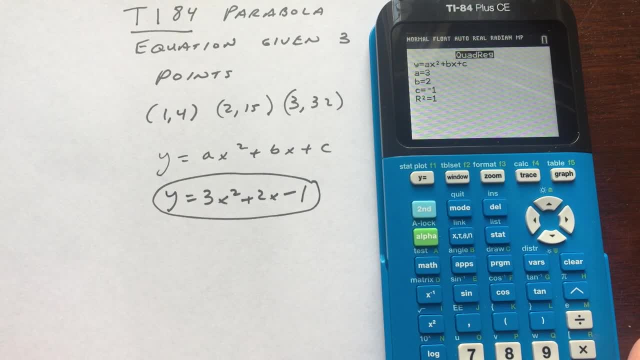 Mario's Math Tutoring YouTube channel. Subscribe to the channel And I look forward to helping you in the future videos. I'll talk to you soon. 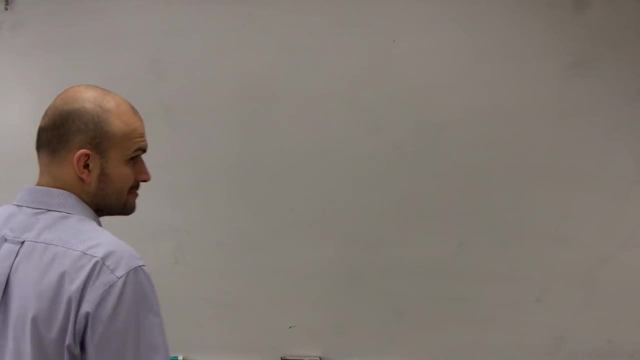 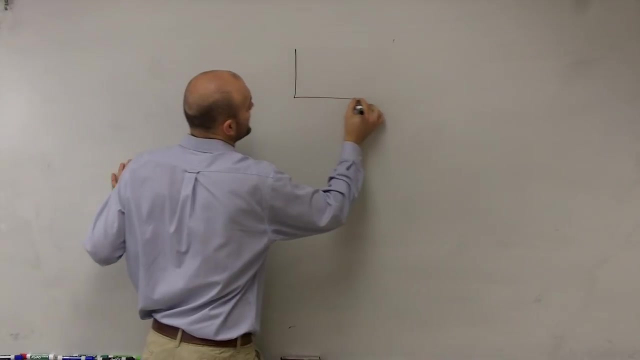 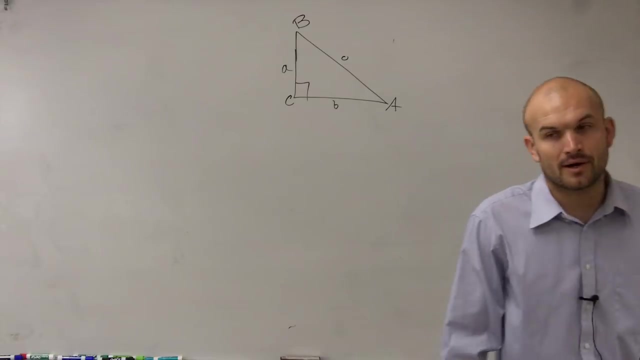 No way. Okay, here we go. So let's go back to our triangle, the one that we love. All right. so if we had this triangle, what I'm going to talk about now is area. all right, So we have a right triangle. You're like: all right, I know, right triangle, that's the same thing.